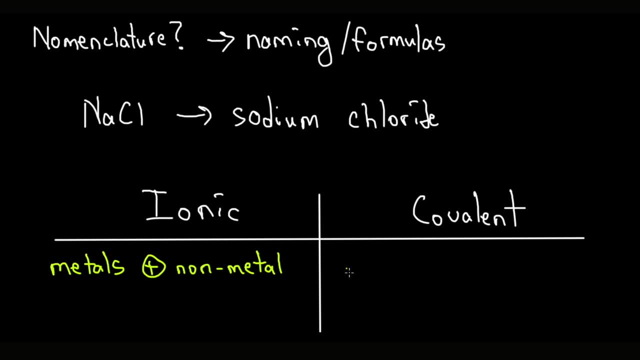 and non-metals, and covalent bonds are going to be between two non-metals. So why am I bringing up this split between ionic and covalent bonds? Well, because the nomenclature, inorganic nomenclature, is going to be different between ionic and covalent compounds, So we need to understand the difference. 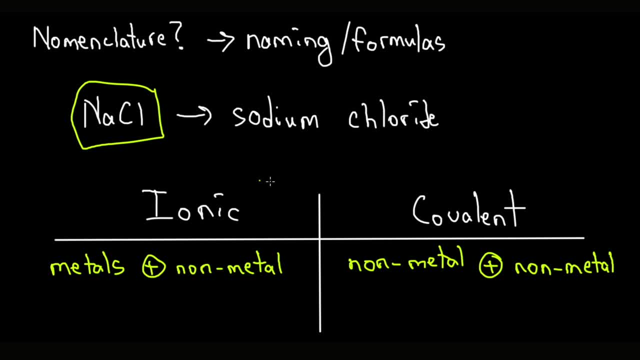 First you need to understand the difference between ionic and covalent compounds. First you need to identify: is this ionic or is this covalent, and from there on we'll be able to go and do our naming of that compound. So first let's discuss ionic compounds, as they involve several nuances. 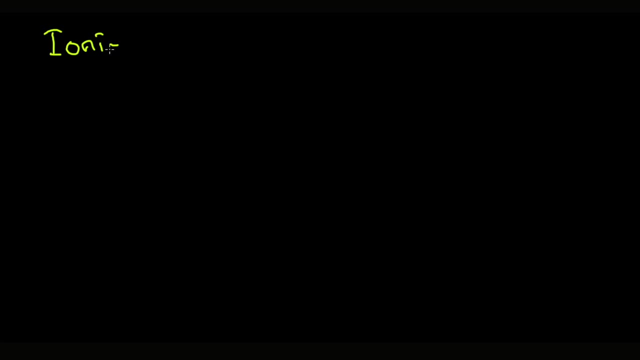 So the naming for ionic compounds is going to be quite simple. You're just going to have your metal name, Then you're going to write your non-metal name, as it specifies on the periodic table. However, you're going to also add an ide ending to the non-metal. For example, if we have NaCl, 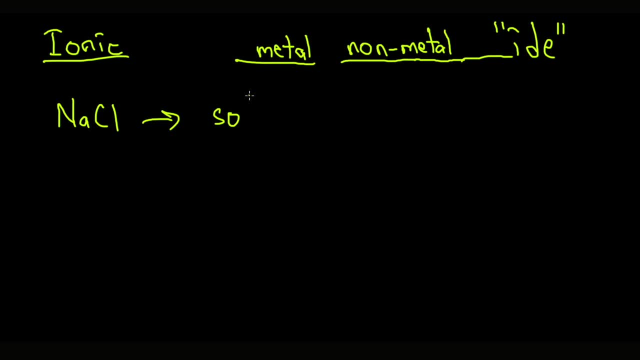 as we mentioned, the name is going to be the metal, which is sodium, as it says on the periodic table. No changes there. Then it's chlorine. However, instead of writing chlorine i-n-e, you're going to substitute the ending with ide and now you're going to have sodium chloride. Another example would: 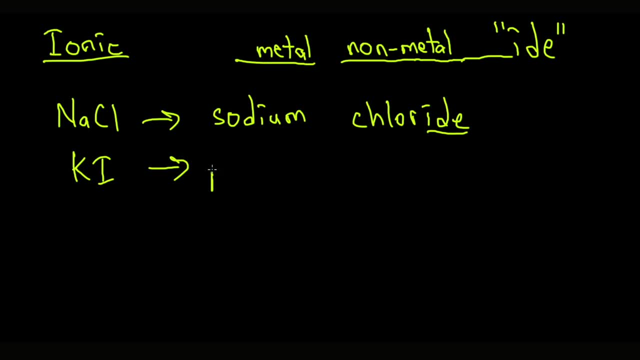 be Ki. So we have potassium as the metal- We just write potassium- and we have iodine- iodine as the non-metal. However, we know that we have to replace ine with ide, and now we're going to have iodide. Then we have something like CaF2.. Now the name of that is calcium, If we're looking. 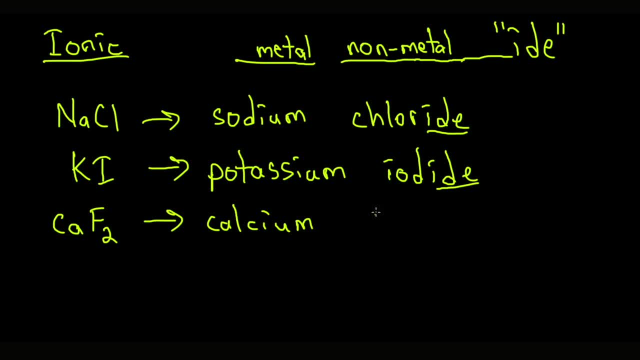 at the periodic table, and non-metal is going to be fluorine, but it will become fluoride as the name changes to ide. Now this stays pretty consistent throughout. so these are the very simple ones. Now, if you're wondering why i have a 2 over here, we are going to have to now. 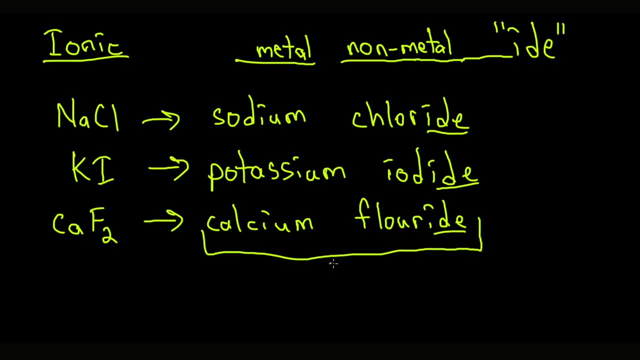 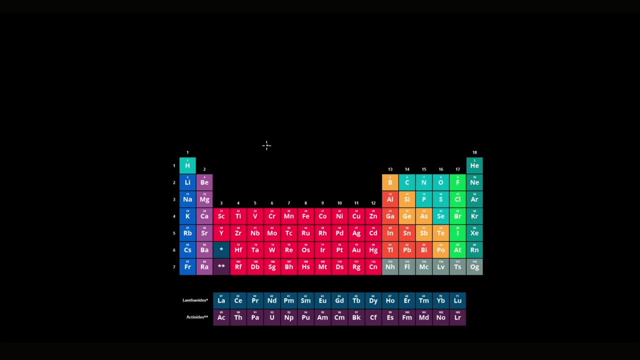 learn how to go backwards from the name, backwards to the formula, and in order to understand that, we have to take a look at the periodic table. So, in order to understand how to go from the name to the formula, we have to understand charges, Charges of different groups on the periodic table. This is something that we've discussed previously. 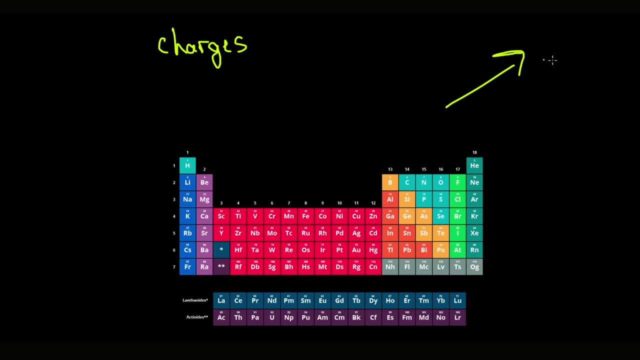 on in another video and i'm going to link that right up here so you can check that out if you haven't seen it yet. That knowledge is required in order to understand the rest of today's lecture. So here, what we have is: we're just going to. 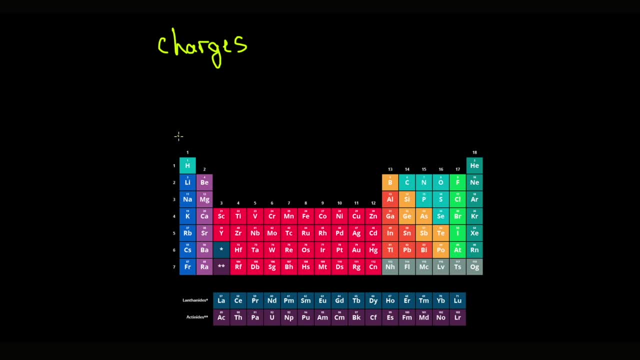 have to show the charges of the common groups and i'm not going to explain how they happen. You will have to check out that video that i made previously, just for the sake of time. Here we have a plus one charge on the first group, plus two charge on the second group. 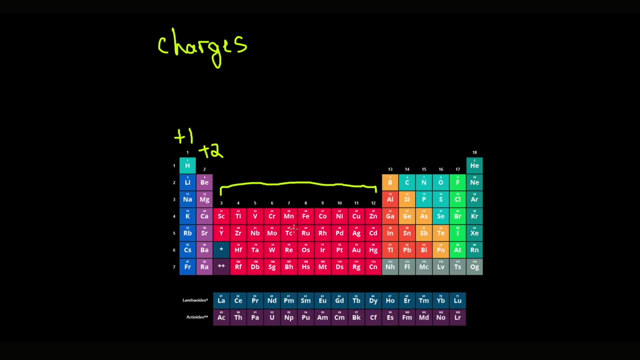 Transition metals are going to be multivalent, which we are going to talk about a little bit later. The third is going to be plus three. Here we'll have plus four or minus four, depending the situation. then for the non-metals, starting with nitrogen and phosphorus, 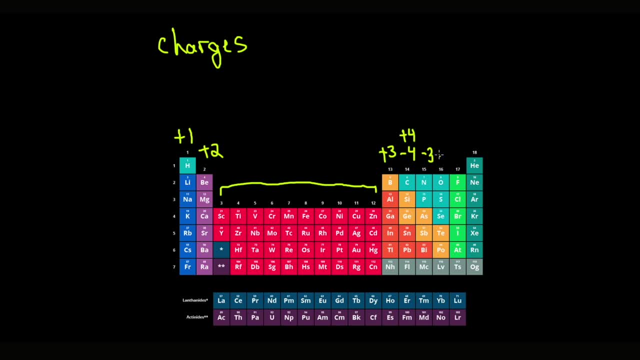 here we're gonna have minus three: oxygen, sulfur, selenium- negative two, and the halogens- fluorine, chlorine, bromine, iodine- are gonna be negative one charge and, of course, the noble gases do not have a charge. so these are the charges that we should know if we want to make the formulas. so let's take a look at. 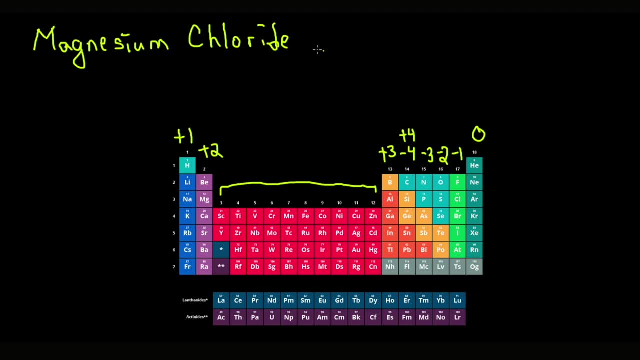 some examples. so if I have magnesium chloride, what we're going to do in order to make the formula is: we're going to do a crisscross method, so we're going to write out the ions for each of the elements. so magnesium is right there. so 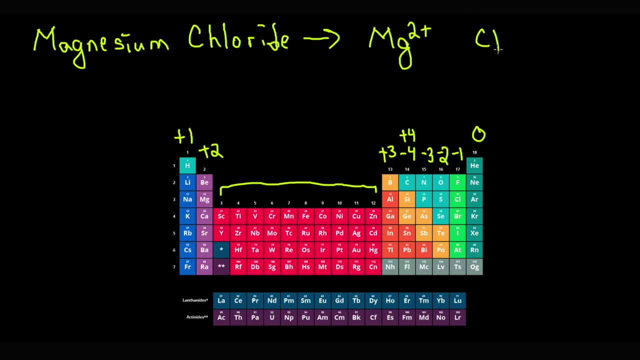 it's ion is going to be two plus, and chlorine is right there, so it's ion is going to be minus one. now all we're going to do is we're going to crisscross the negative. one charge will go down to one as a subscript for magnesium, and the two is going to go down as a subscript. 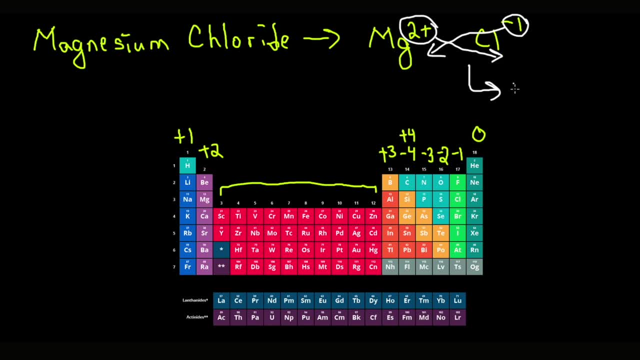 for chlorine. so therefore our final formula is going to be mg1, but we're not going to write a subscript of one cl2. so we're going to include all the subscripts except one. we just assume one is obviously there. so what this really means is I have one atom of magnesium and I have two atoms of. 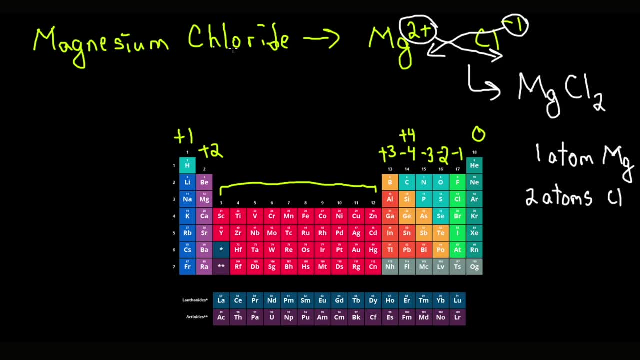 chlorine in one compound of magnesium chloride. next, let's do lithium oxide. lithium is right here, element number three. so it's going to have a plus charge and oxygen is going to have a two minus charge. if you crisscross them, we're going to get Li2O. and another example: we have potassium. 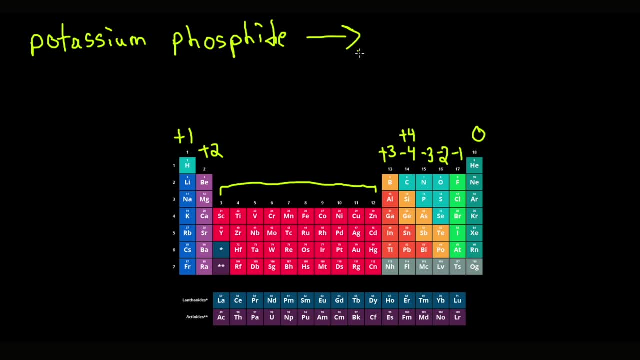 phosphide. so here, if we are going to do the ions, potassium is K plus and the ion of phosphorus is P3 minus. when we crisscross we're going to get K3P. now, remember I mentioned that ionic compounds nomenclature is going to have a couple of nuance, meaning there's a 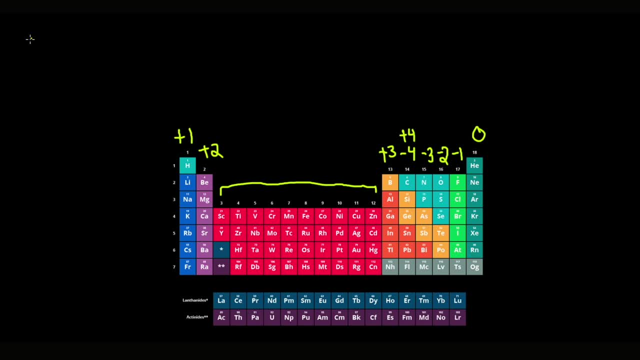 couple of strange cases. so the first strange case is going to be with the transition metals. so the transition metals are right here on the periodic table. so it's this block of these elements, and the reason why they're going to have a nuance is because some of them are multivalent, and multivalent means they're going to 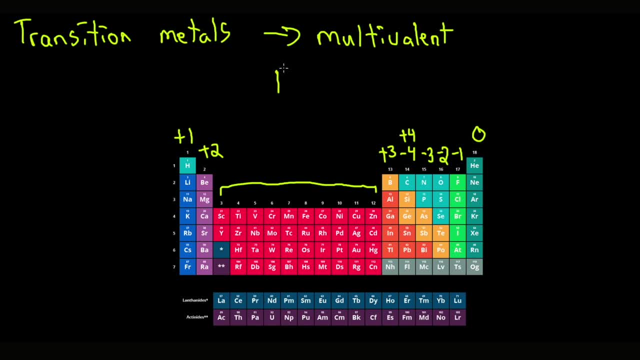 have multiple charges. so, for example, something like iron could be iron 2 plus or iron 3 plus. another common one is copper 2 plus or copper just plus, or we could have a lead PB two plus, or we could have lead 4 plus. so when we are encountering the situation, 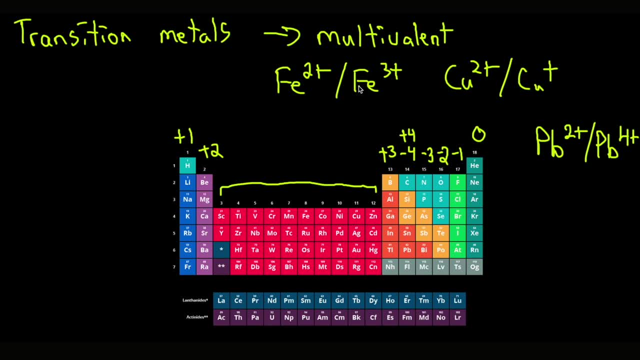 and somebody says, okay, we, we've got iron oxide. we don't really know what the formula is because we don't know what iron you're talking about. so we have a problem with this nomenclature, the rules that we have used so far, because, if I 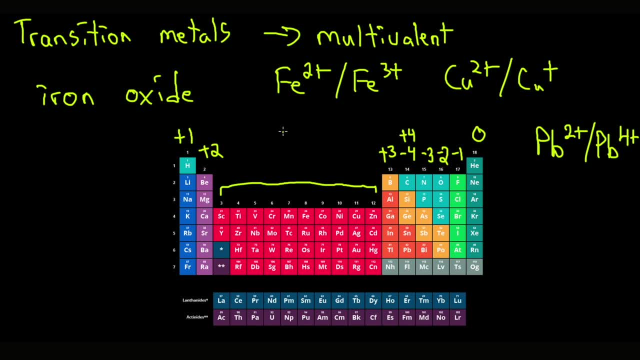 just put down iron oxide. I don't know what the formula will be, since I don't know which iron where I'm using, In order to omit this problem. there is a scheme to do so, For example, if I am talking about Fe2O3,. so this is my formula and I want to do the name of this. 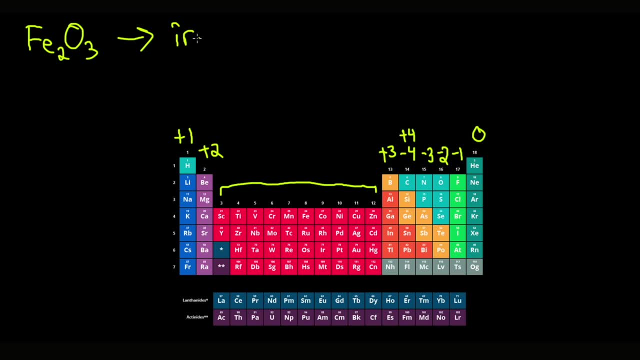 I would have to indicate what is the ion for the iron. So here, if we split these backwards, if we do the crisscross backwards, Fe is going to be 3+, because the 3 is now going to go up here. 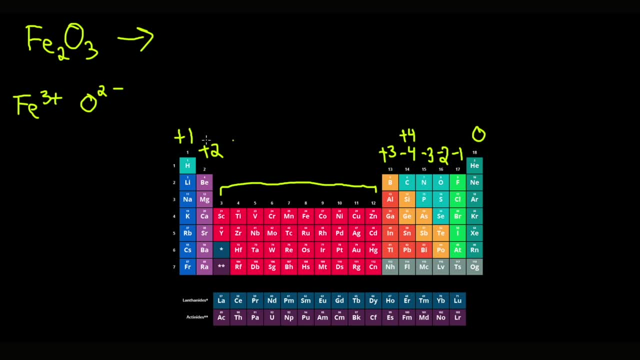 and oxygen is, of course, 2- and that's not going to change because oxygen is not multivalent. So it is going to be the iron with 3+ charge. In this case, we're going to have to write iron and we're going to put three Roman numerals in brackets. 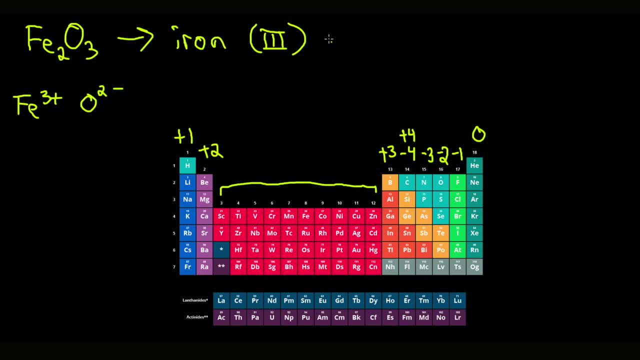 to indicate that it's iron 3.. And here we're going to have our oxides, So the rest of the naming is going to be exactly the same. Another example will be FeO and the name of this, so, since we're going to have Fe2+ and O2-, 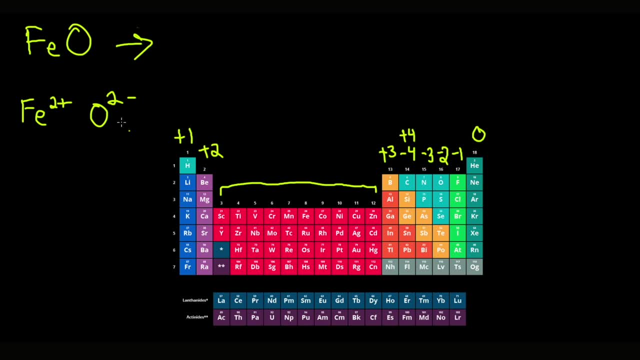 I'm going to explain why there's no subscripts here. You might be wondering like hey, what's going on? We should have some sort of subscripts 2 and 2.. However, we don't put the subscripts because they're simply going to cancel out. 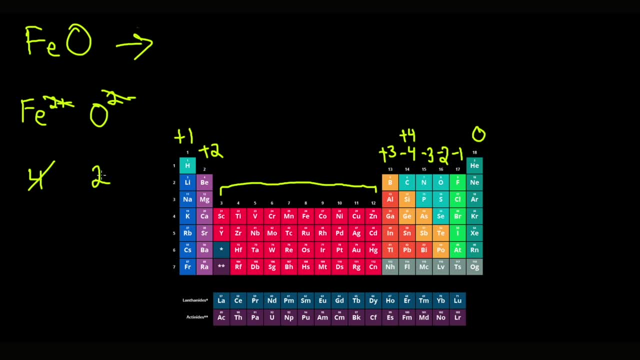 So if we have 4 and 2, well, that's going to cancel out and this will just be 2.. So these charges are going to be cancelable. therefore, our subscripts will remain as 1 and 1.. 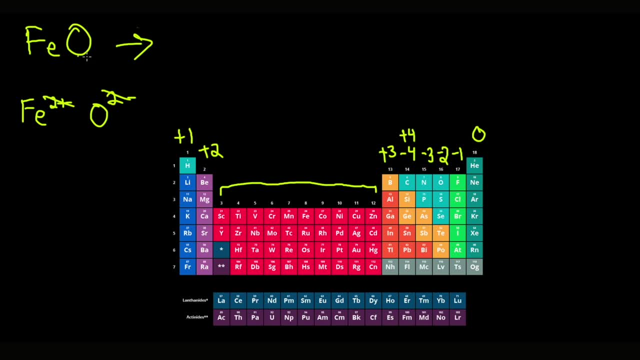 Now, for that case, we still have to indicate which iron it is. We do not have iron 1, and we do not have oxygen with a negative charge. We have oxygen with 2 negative charge. So in this case we would have to indicate this iron, which will be iron, and Roman numerals 2,. 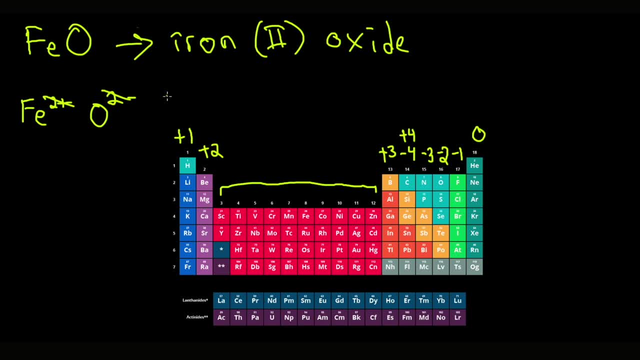 oxide, and that's the name of FeO. Another prominent example of cancellations is going to be here with PbS2.. So, as I mentioned earlier, lead- which is right here- is also multivalent, and it could be lead 4+ or lead 2+. 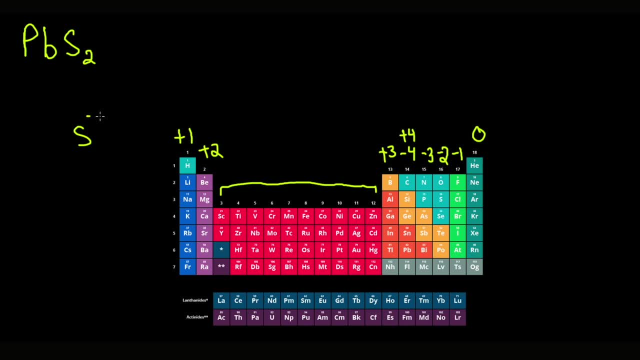 And in this case, we know that sulfur is minus 2,. since sulfur is right there And since this is the arrangement, I know that lead is 4+ and I'm going to explain a little bit how that works. Again, we're going to have the cancellation. 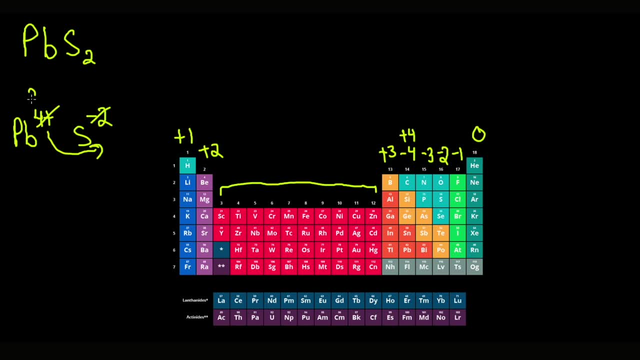 since it's 4 and 2, and these both divide by 2, this becomes 2, and this becomes 1.. So the 2 goes here and the 1 goes there, and that's why we have this sort of arrangement. 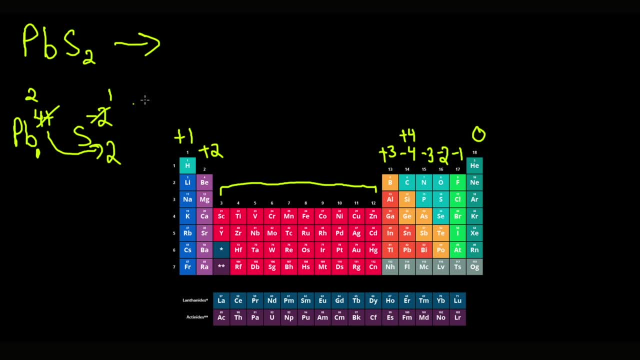 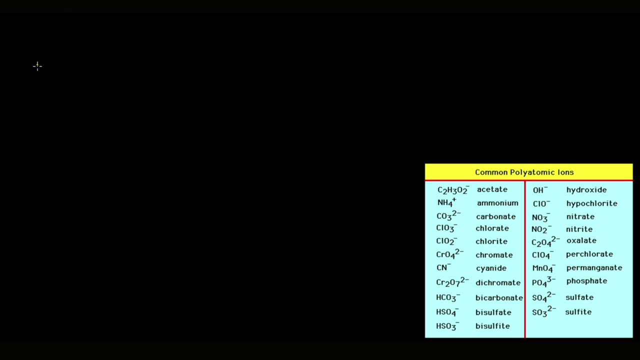 So we still have to indicate that this is lead 4+, So we will write lead, Roman numerals 4, sulfide is going to be the name of this compound. Moving on to the second nuance and this is going to have to deal with polyatomic ions, 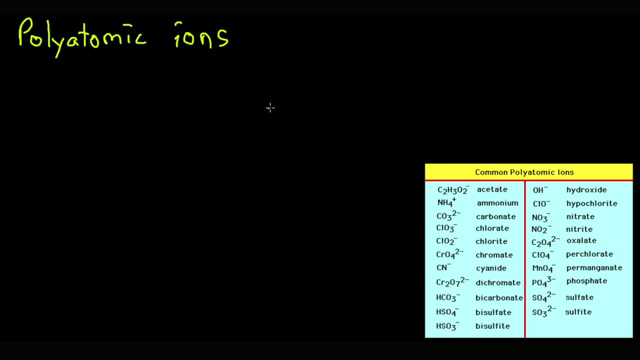 You might be wondering what polyatomic ions are. Well, poly means many, atomic means atoms. so many atoms, ions. So typically, when we talk about ions, previously we just had one element which had one atom And we would have its ion like Ca2+. that's just one element. 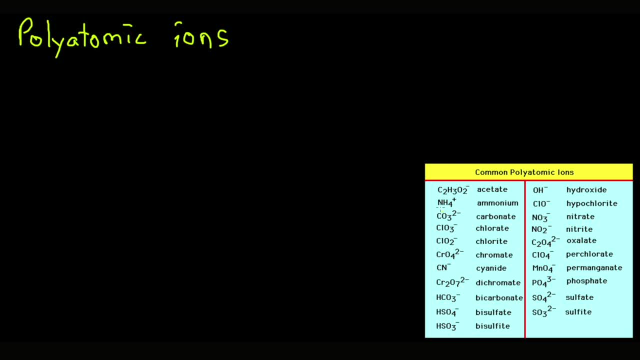 However, in this case we're looking at specific polyatomic ions, which will have multiple atoms and multiple elements, in most cases connected together to make an ion, And these, most of these, the ones that are negatively charged, are going to act as nonmetals and our ammonium right here is. 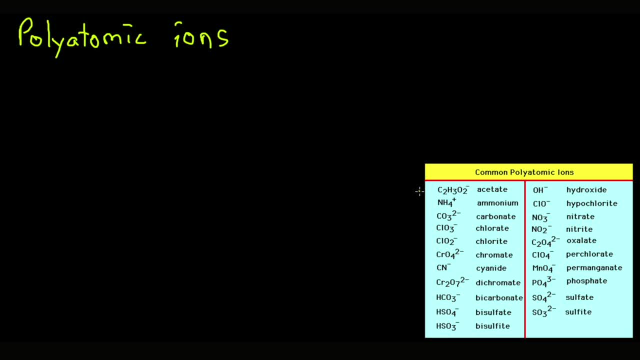 going to be positively charged, So it's going to act like a metal, And when they are bonding with other elements in order to make them stable, they're going to go through ionic bonding. Therefore, the naming is still going to be very similar. 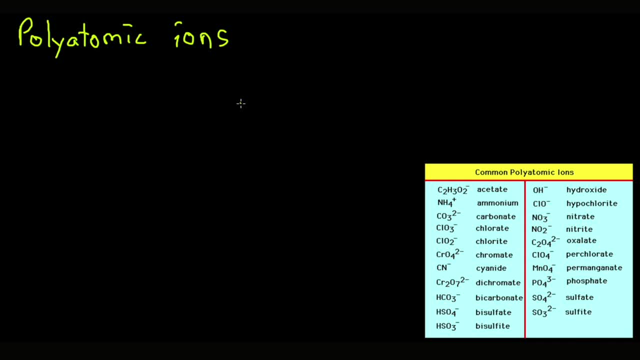 And I decided to include it here with the ionic compounds nomenclature. So let's take a look at some examples of how this works. But before we do that, one thing to know is that when we have polyatomic ions, the I-D-E ending 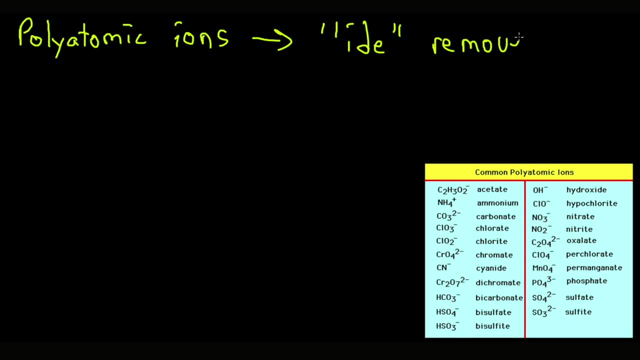 is removed. So, because most of these are going to be acting as nonmetals, they're going to have other endings: 8, I-T, more 8, I-D. some of them will be I-D-E, but the general ending of I-D-E, replacing it with whatever's there, is not going to happen. 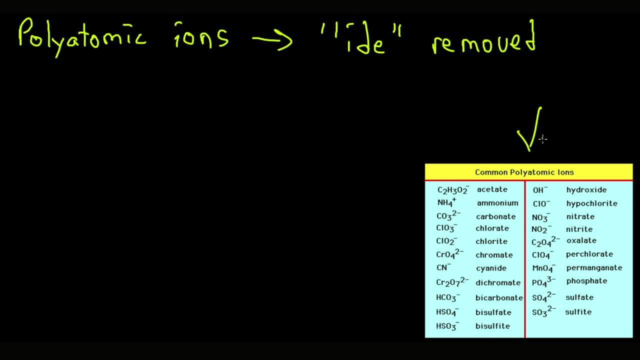 We are just going to keep the name the same of the polyatomic ions. For example, if we have NaOH, I can identify that the OH is going to be a polyatomic ion, Since here it says it's a hydroxide with OH-. 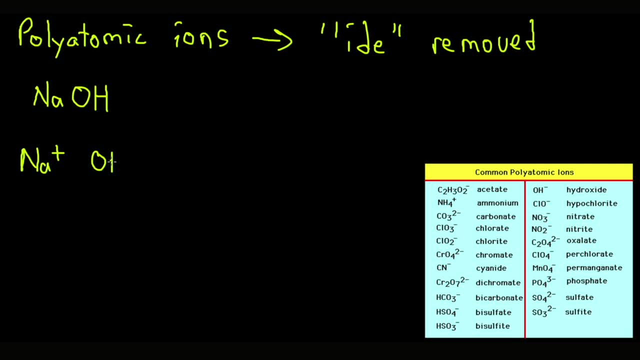 Now I know my sodium has a plus charge, OH- has a negative charge. So when I'm doing the naming again, same thing: metal name is sodium And the hydroxide is going to act like a nonmetal. But I'm not going to replace the ending, since it already has an I-D-E. 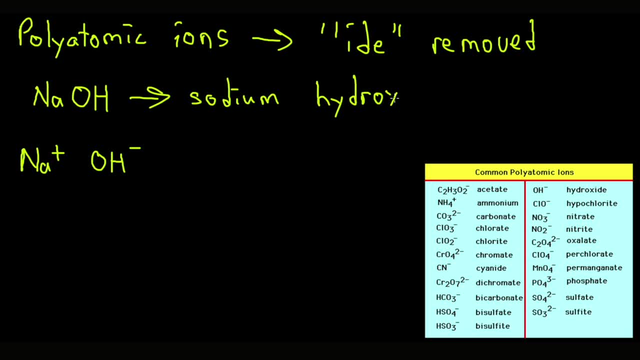 So I will just call it hydroxide. Very simple, since in polyatomic ions you will just write the name of the polyatomic ion without being worried about I-D-E. Another example: let's go backwards. We've got magnesium nitrate. 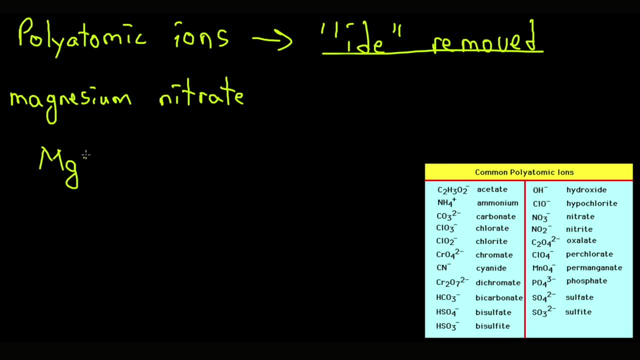 So this should be quite simple. Magnesium- we know from the periodic table- is 2 plus And nitrate, if you look at your table, is 2 plus If you look at your common polyatomic ions chart NO3- that's going to be the formula for that. 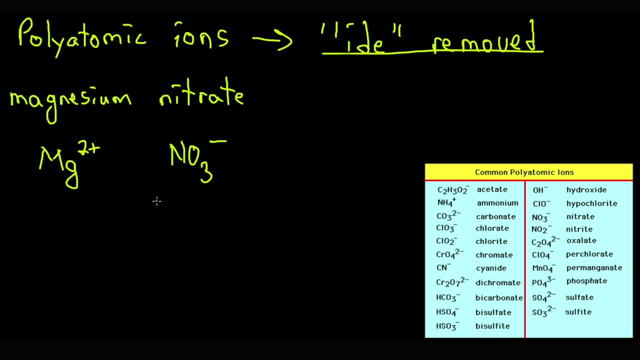 Now when the two connect. this is very important here because it creates another tiny little nuance When these two connect. you see the subscripts. The 2 is going to go here, But we have a problem because it's going to be kind of awkward if we place another 2 there. 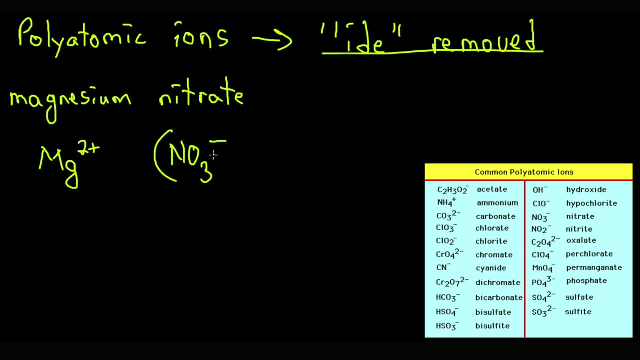 It looks like a 32.. So instead we're going to cover it in brackets And then put a 2,, signifying that we have two NO3s. So let's see how that works in a full formula. So we're going to write our magnesium. 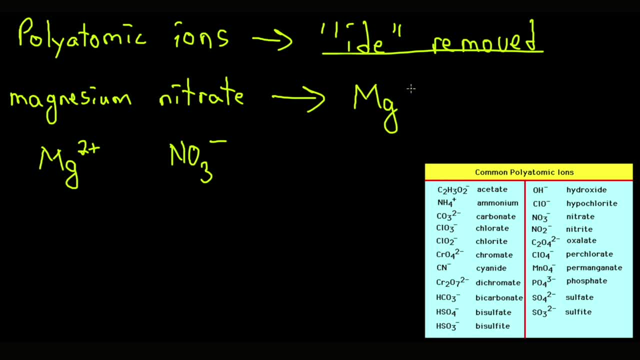 Now this has a negative 1 charge, so it will just be 1 as a subscript. And then we're going to put NO3 in brackets, And then we're going to put a 2 around it, signifying that I have two NO3s and one magnesium. 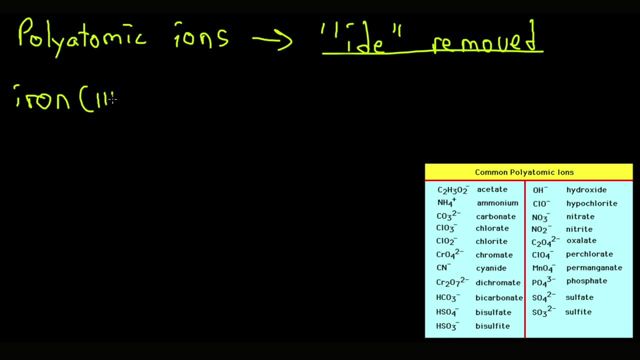 Let's do another example: NO3, chromate. Now here I know iron 3 will be Fe3+ And chromate. when I'm looking here it's going to be CrO42- so that's right there. And when we connect the 2,, the 2 and the 3 are going to exchange. 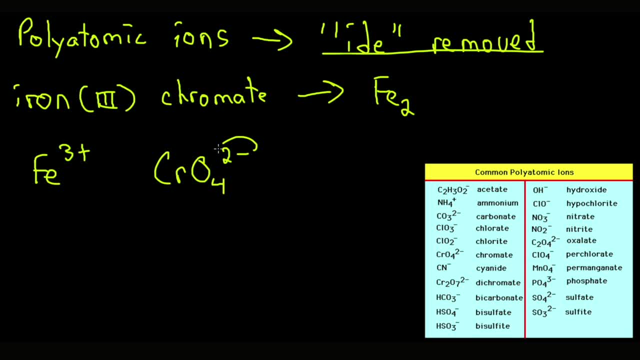 So I'm going to have Fe2 as the subscript because of the charge of chromate, And for chromate I'm going to put it in brackets, CrO4 in brackets And the 3 will go outside of it, indicating that I have 3 chromates and 2 irons in this compound of iron: 3 chromate, 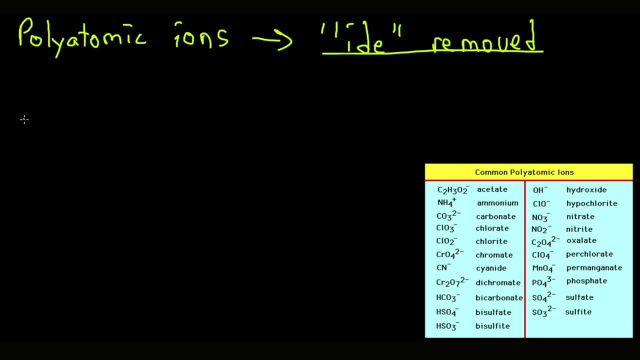 And finally, let's take a look at our ammonium phosphate. So here, I know that ammonium is going to be NH4+, So it's going to act like a metal, And the phosphate- which is right there, is going to act like a nonmetal, since it's negatively charged. 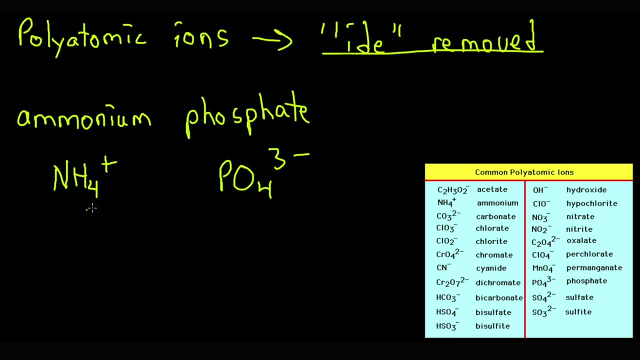 PO43- Now, when these are exchanging their charges, when we do the crisscross we end up with NH4 in brackets 3 outside of it, to indicate we have 3 NH4s And we have 1PO4. 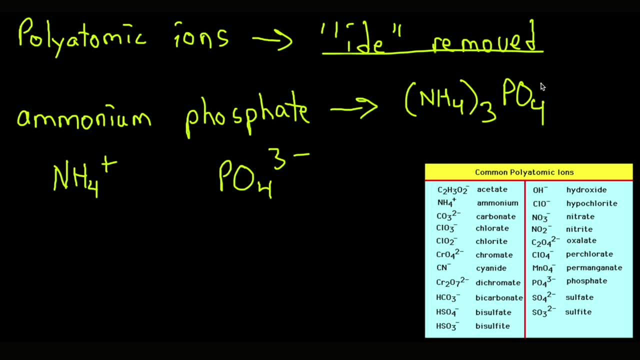 And this will not be in brackets, since our subscript is just 1.. Now, if you were to determine how many atoms we have, so let's do that. If I am looking at this, I know that I have 3,, 3 ends. 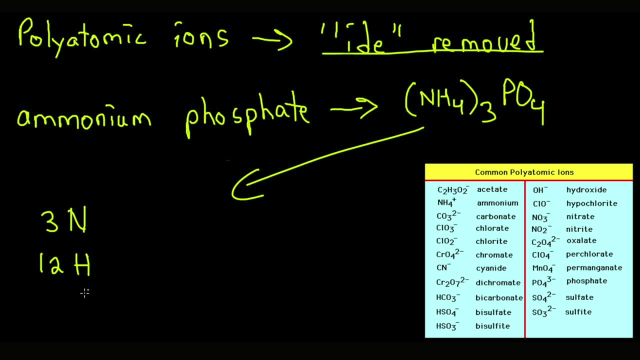 I have 12 hydrogens, I have 1 phosphorus and I have 4 oxygens. How did I know I have 3 and 12?? Well, because I can just take the 3 and multiply it inside of the bracket. 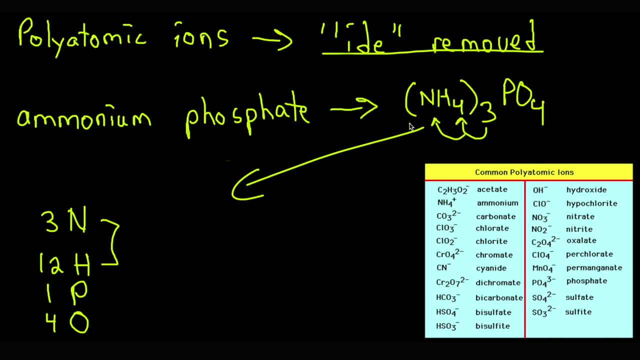 Just like you would have done when you are doing simplification in math and you're opening up the brackets. So essentially, the 3 will multiply inside. The subscript of nitrogen is 1. And the subscript of hydrogen is 4.. So 3 times 1 is 3.. 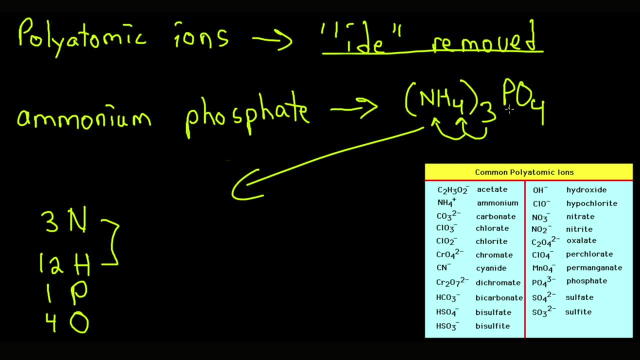 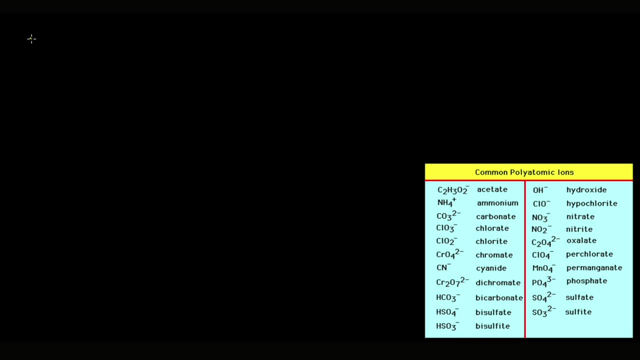 3 times 4 is 12 for the hydrogen. Now here we just have the 1 phosphorus, since it's the 1 subscript, And oxygen will have a 4 subscript, so 4 oxygens. Now another thing to consider is how we are going to talk about our acids and bases. 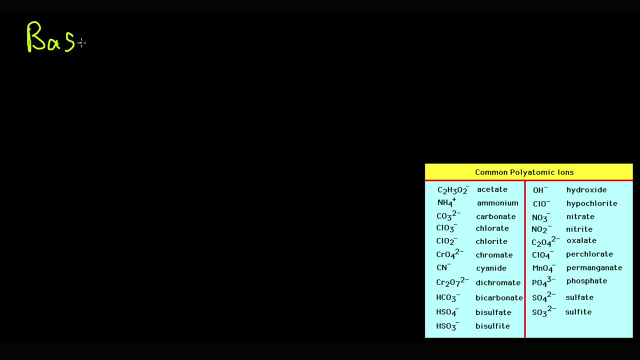 So bases are going to be simply named normally as our regular inorganic nomenclature. that we have done already. However, acids are going to have special names And here are some rules for naming acids. These blanks are going to signify the nonmetal. 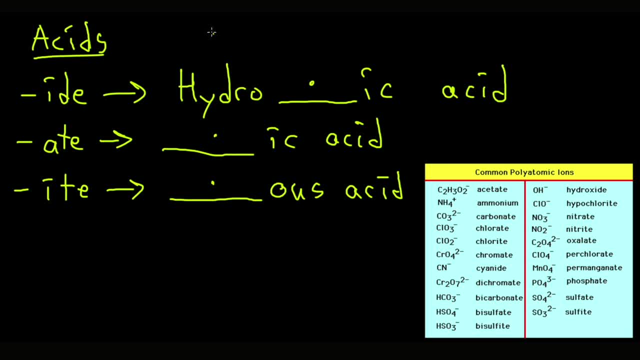 So here, nonmetal, nonmetal, nonmetal name, And you're going to get your acid. So let's take a look at some examples. If I have HCl, then my inorganic nomenclature name is just going to be hydrogen chloride. 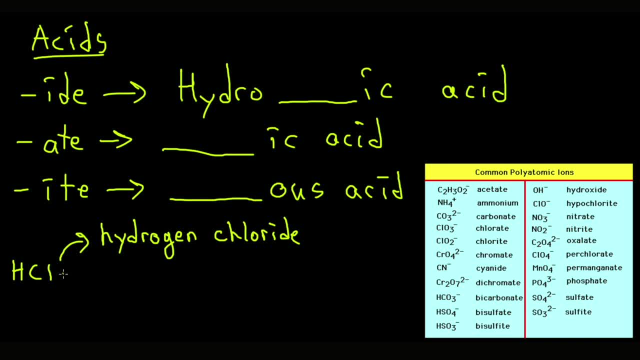 However, if I am naming it as an acid, the acid name is going to be hydrochloric acid. As you can see, here we have our chloric, meaning our nonmetal. that would go right there. We put a hydro in front and we end it with ic acid. 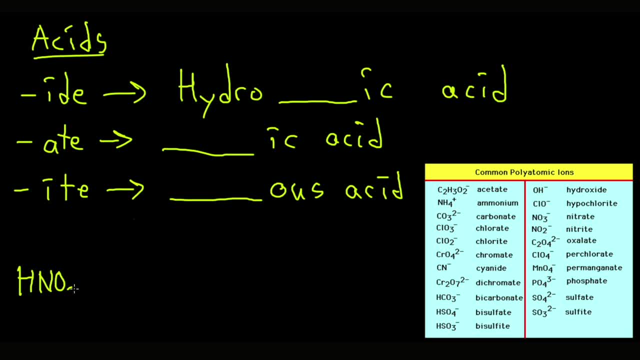 Another example: if we have HNO3, the name of this is going to have the polyatomic ion With the inorganic nomenclature And we're going to have hydrogen nitrate. However, if we are naming it as an acid, 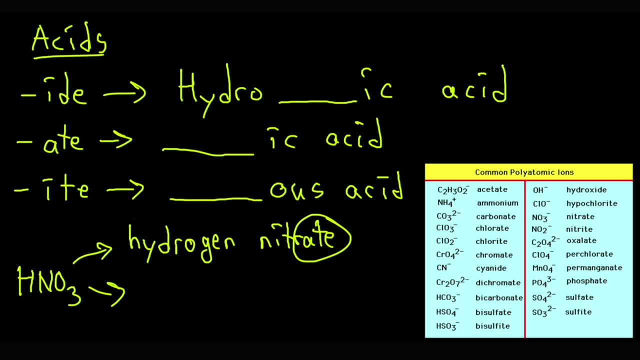 this has the ending of 8 right here. So the ending of 8 is going to have its nonmetal ic acid And the nonmetal is going to be nitrate, So nitric acid will be the name. And finally, if we have HClO2,. 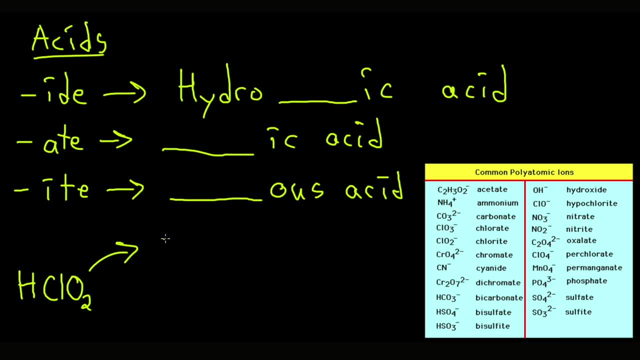 the name of this is going to be hydrogen chloride, Chlorite, right here, ClO2-. Now we know that chloride will turn into oos acid, So the nonmetal is chlorine, So the name of the acid is going to be chloris acid. 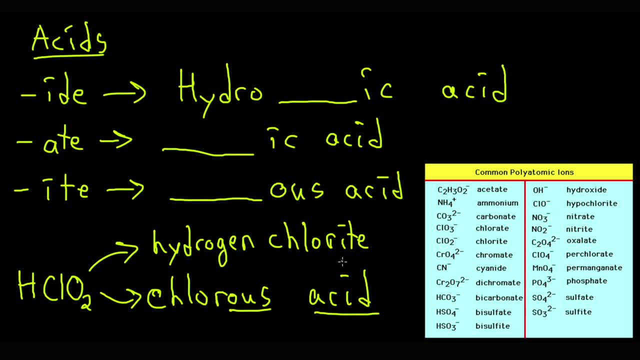 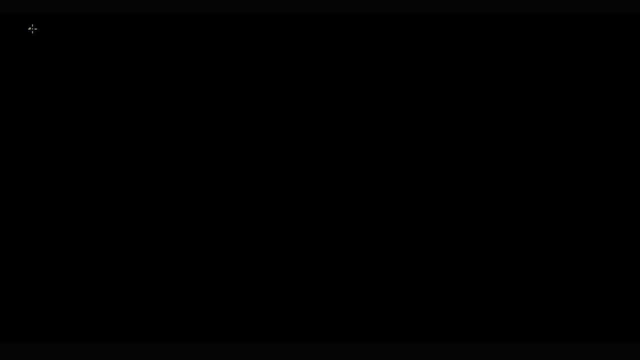 So you can see, here we add the OUS acid as the ending. So now that we're done with ionic compounds nomenclature, now let's talk about covalent nomenclature, And I saved this for last, because it is really a lot easier than ionic. 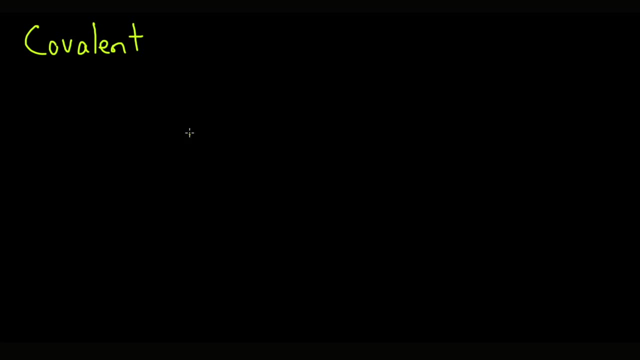 It does not have nuances really. So what this includes is going to be prefixes. So prefixes are words or parts of words that come before the main word. So what these represent is: if you have a subscript of 1, you're going to put mono. 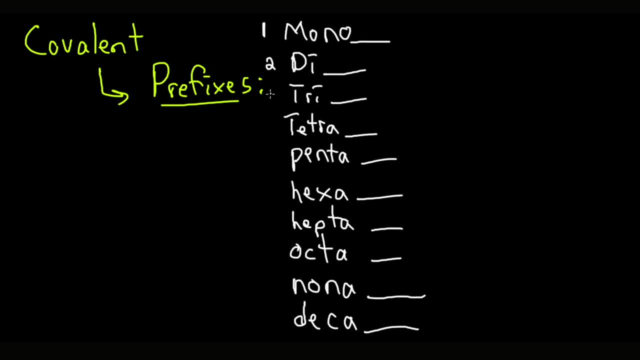 If you have a subscript of 2, you'll put di. If you have a subscript of 3, you'll put tri in front of the metal or the nonmetal. So the only exception to the rule here is that when you are doing your naming. 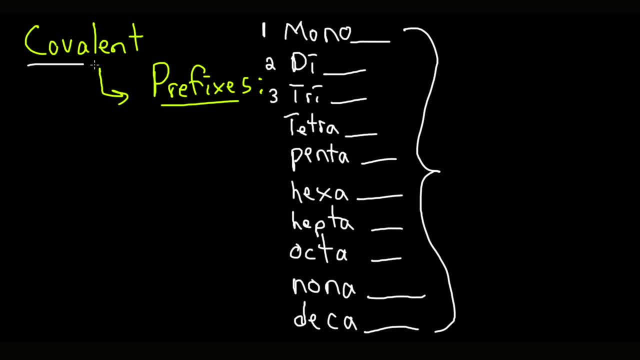 the first element, because covalent bonding is going to be between two nonmetals. but the first nonmetal that will be stated mono will be excluded. So let's take a look at some examples here. If we have CO2, we know carbon is a nonmetal. 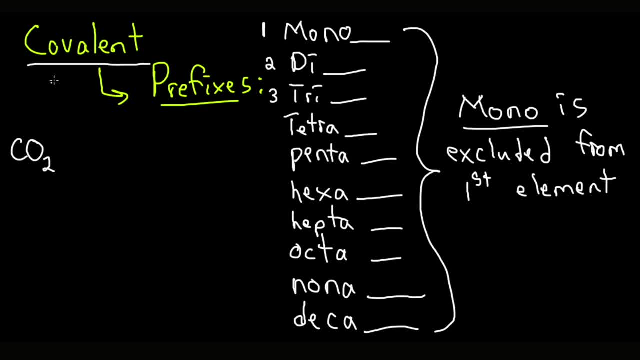 Oxygen is a nonmetal and the two combining will make a covalent bond. So the naming of this is going to be just carbon dioxide And, by the way, as you can see, we still keep the ID ending, as we do with ionic compounds. 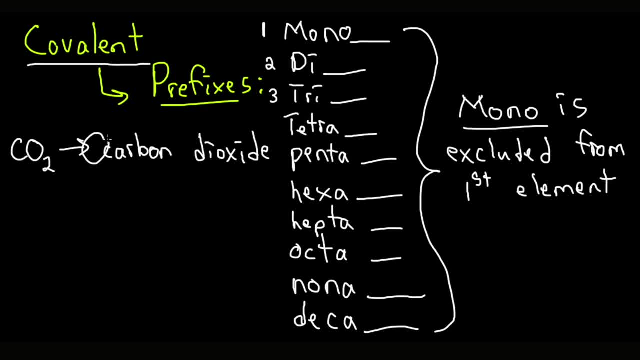 And, as mentioned, mono is not going to go here in front of the carbon, because that's the first element. The first element does not include the prefix of mono. It includes all the other prefixes, but not mono for the first element. So let's take a look at another example here.